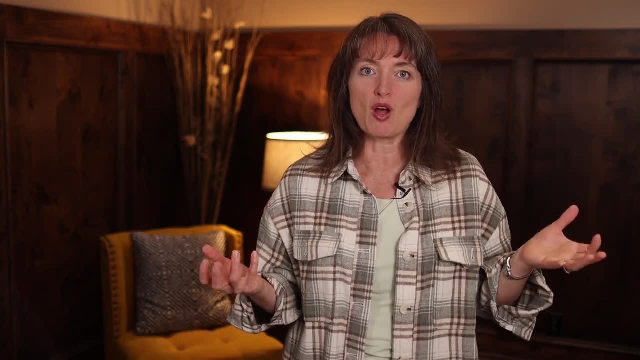 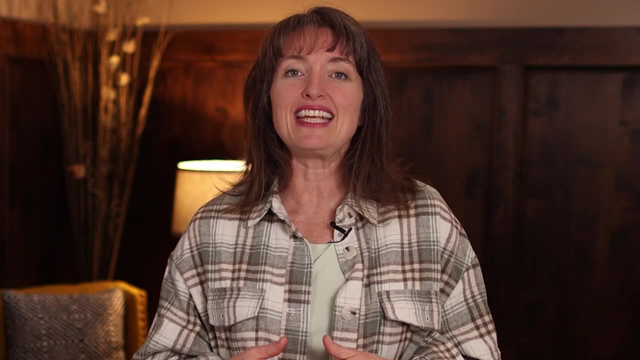 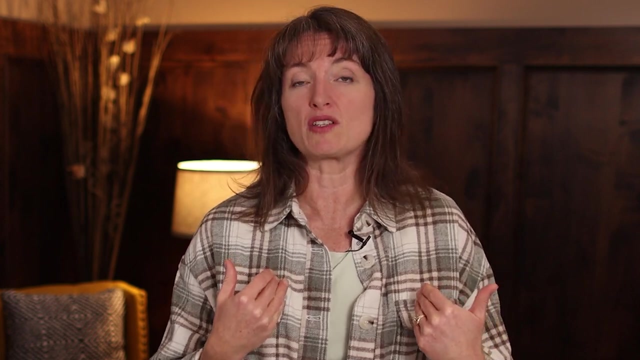 children were constantly needing me and having tantrums all of the time for every little thing I was going to get wiped out. So I had to start teaching everyone time management and following through with it, which for me was kind of a big deal because I wasn't great at time management. I had to teach them how to. 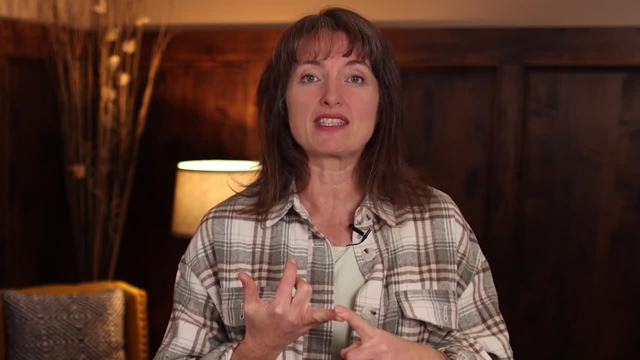 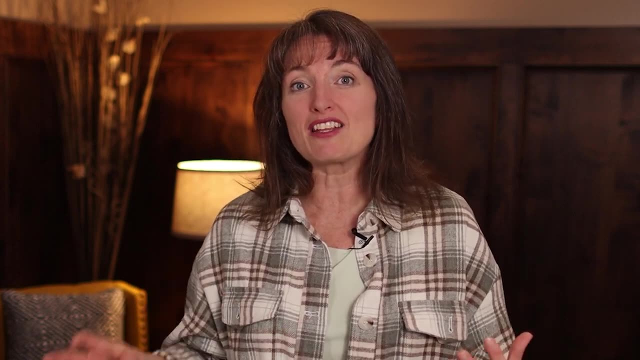 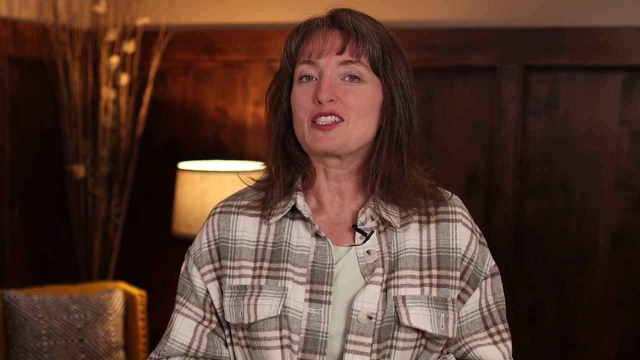 follow through with it, And I also had to teach them the skills that they needed for success. Now, lucky for me, the skills that the foster children and my little children needed to learn to manage their time and to solve their behavioral problems were the same. So what were those skills? That's what we 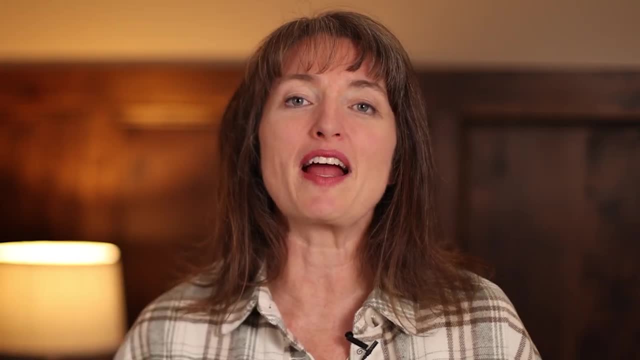 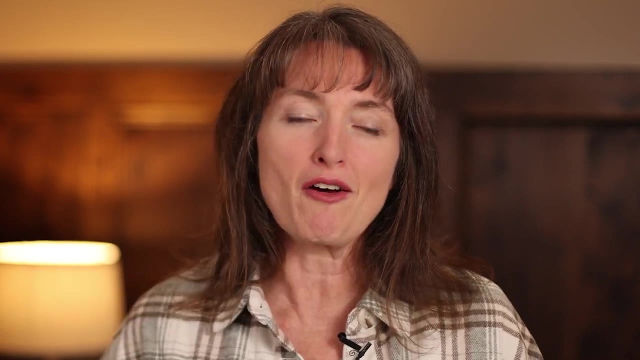 want to talk about right Now. I'm going to share those skills with you, But before I do, click the subscribe button to this channel. When people subscribe to the channel, it allows more people to see the channel, And this channel is all about. 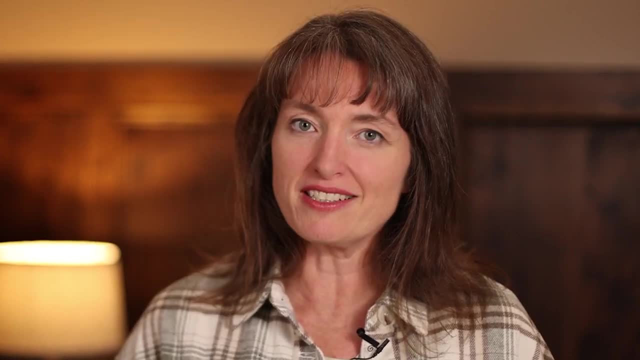 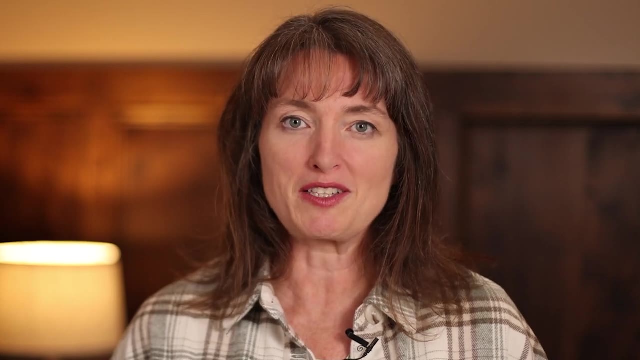 helping families be happy in these hard times where their stress and anxiety and troubles galore. We don't need to have the troubles in our home. We can fix those and I want to help, So click subscribe now. Alright, let's talk about. 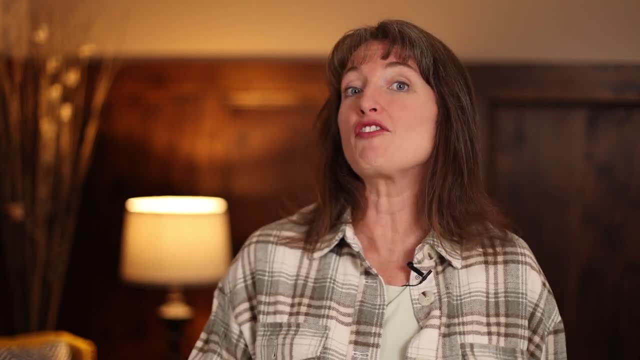 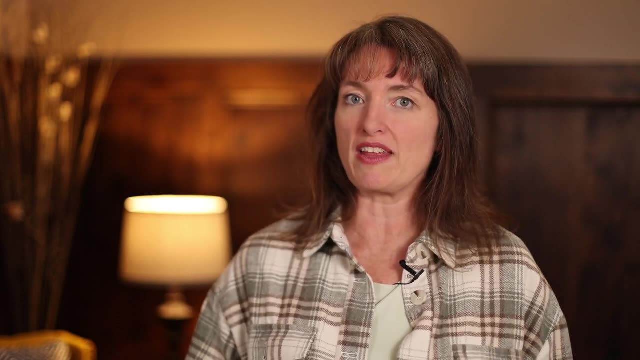 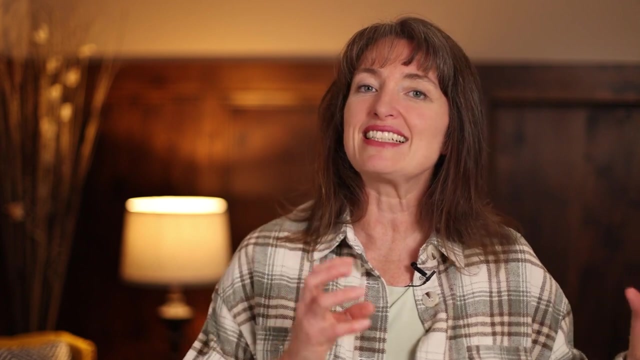 some of the skills that you can use that will help solve behavioral problems, but they also solve time management problems. And then I'm also going to share with you some structural things that you can put in place to help your child learn to manage their time. Once they have the skill, then they can deliberately decide. 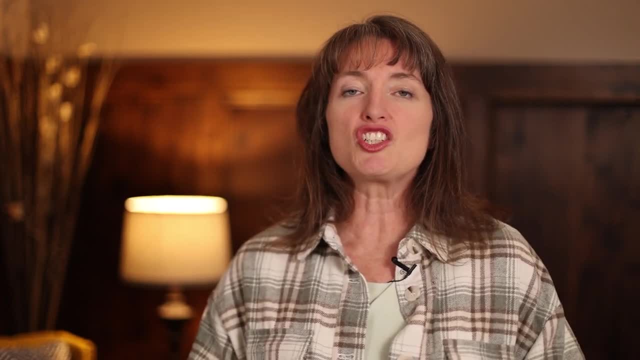 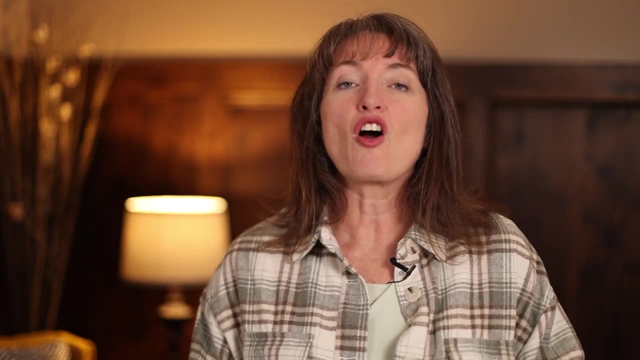 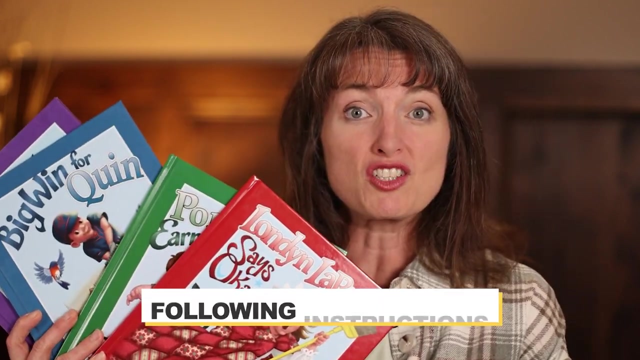 to manage their time. Okay, so the skills that children need to learn for time management, as well as for behavioral problems, are what I call four basic skills. These children's books each teach one of the four basic skills. They are following instructions, accepting no answers and. 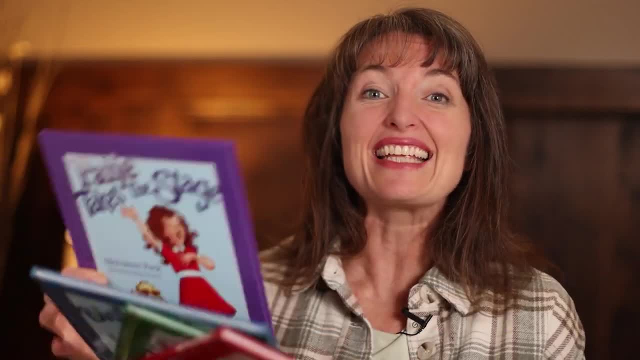 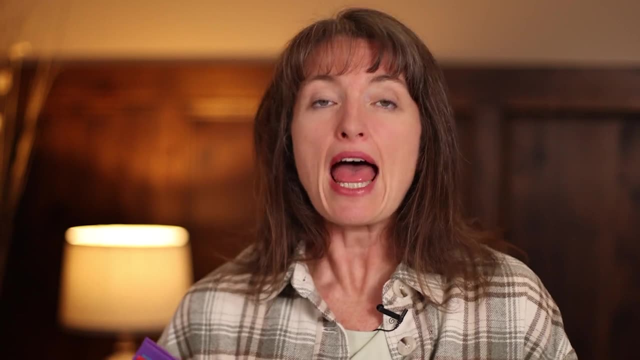 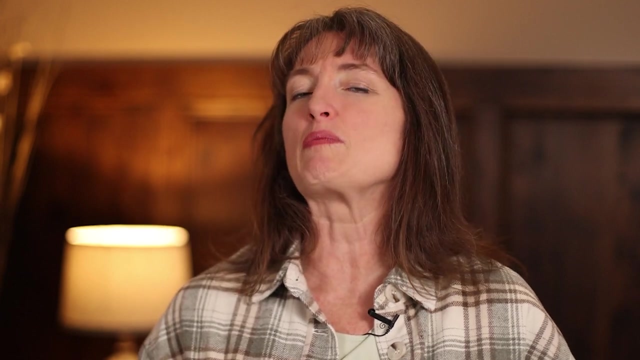 criticism, accepting consequences and disagreeing appropriately. When a person learns all four of those four basic skills, that takes care of 99% of all of their behavioral problems. Honestly, I didn't really believe it at first, because I got told that by the treatment facility that I was working in. 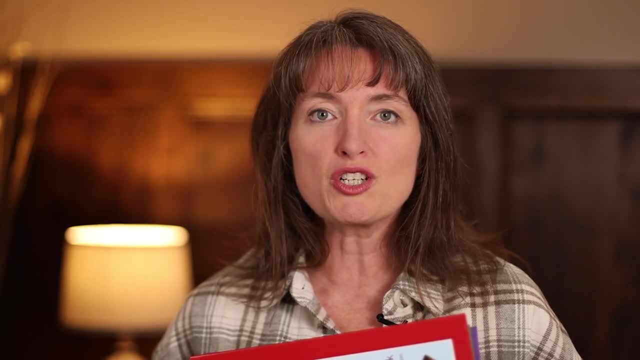 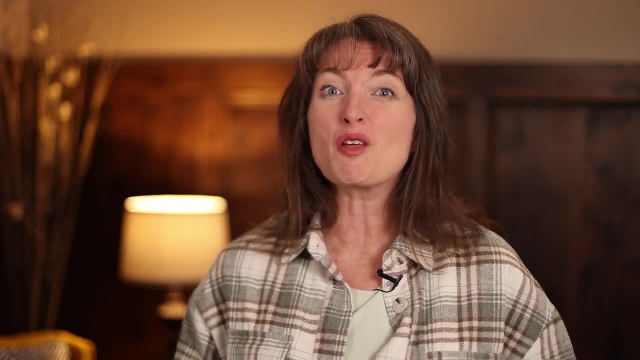 conjunction with. But sure enough, it was true, All of the foster children that came to my home were able to handle all of their problems, for the most part, with these four basic skills. Now I know these books are more geared for children ages 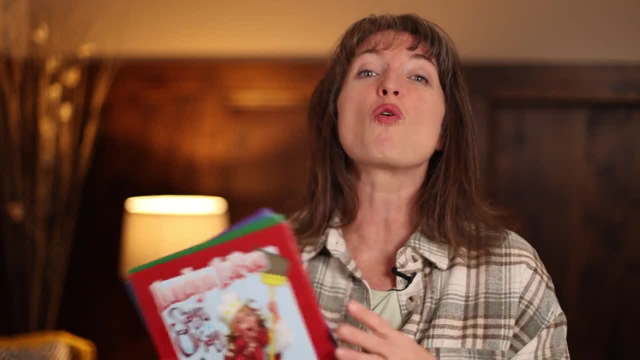 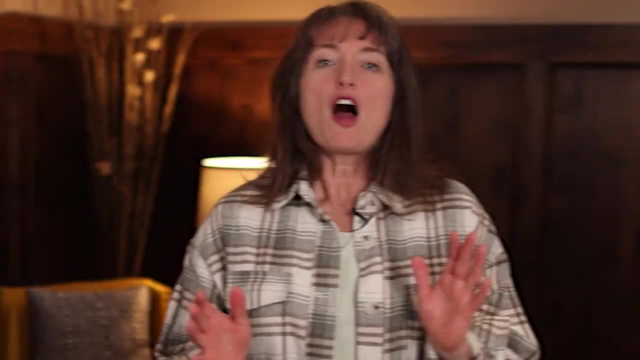 like 12 and under, but the skills are for everyone And you can find those skills in my course, the TSG parenting course on teachingselfgovernmentcom. Alright, so let's talk quickly about these skills, because we have to have a basic understanding of them so that we can. 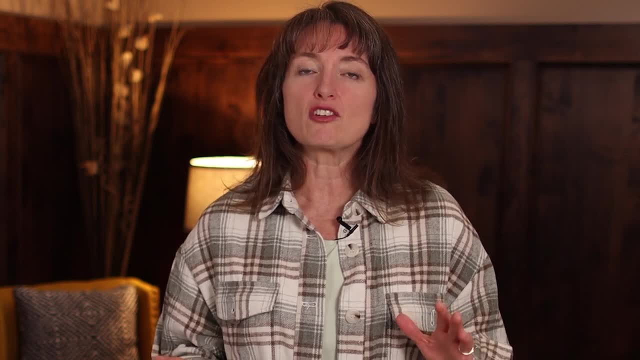 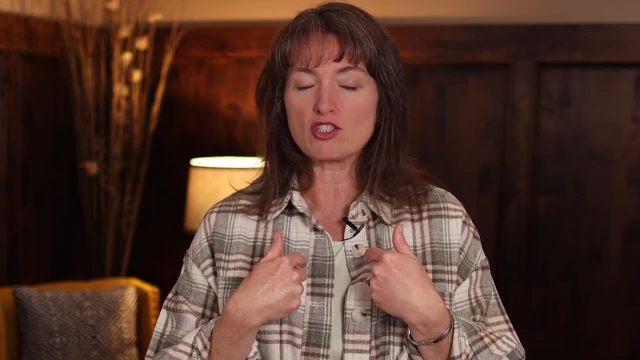 understand time management Now. first off, we need to understand self-government. When a person has self-government, they understand cause and effect and they understand their own behaviors. So you want to teach your children how to analyze themselves, make goals or plans for themselves and then follow through. 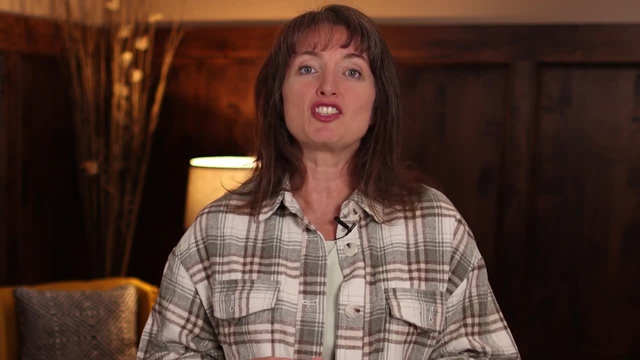 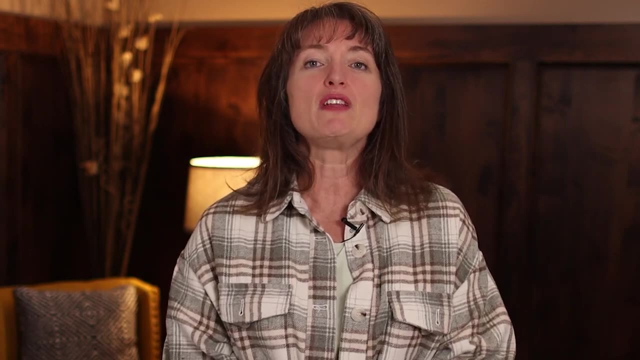 But they won't be perfect at first. In fact, you are going to have to do a bit of hand-holding at first so that they understand what they are seeing in their own behavior. This means that you need to do correcting, praising and, of course, 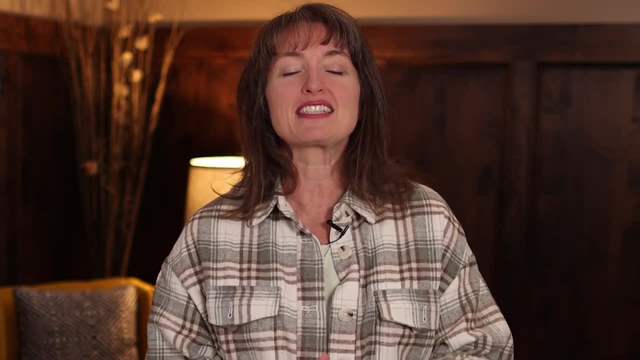 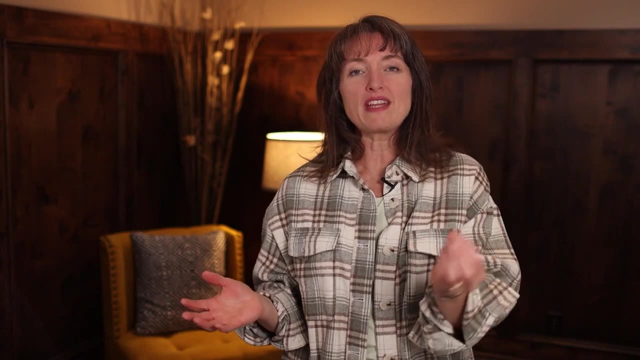 pre-teaching, Because when you pre-teach your children ahead of time, this gives them the best chance at success. I pre-teach my children the 4 basic skills and then I pre-teach in the moment when they need to use one of the 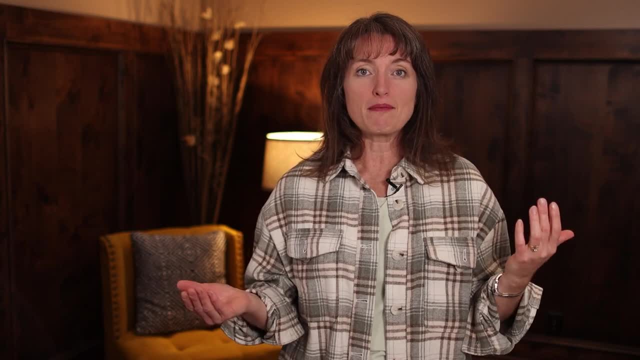 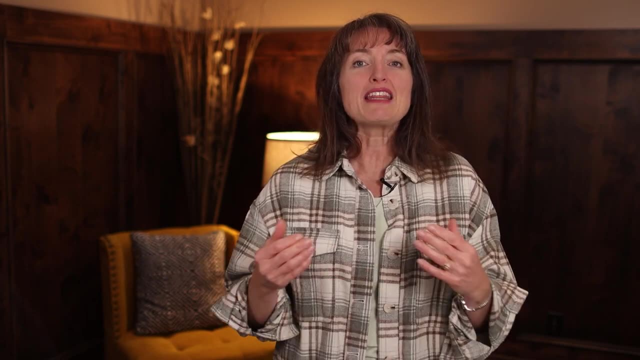 skills. And then, when they use the skill, I praise them to tell them exactly what they did well, or I correct them to let them know it didn't go right and how they can fix it for the future. And in the middle of that correction, we actually 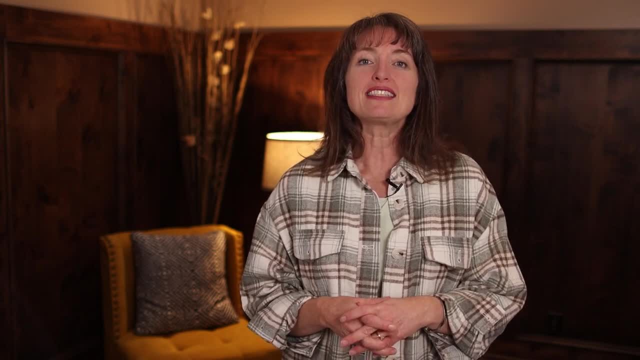 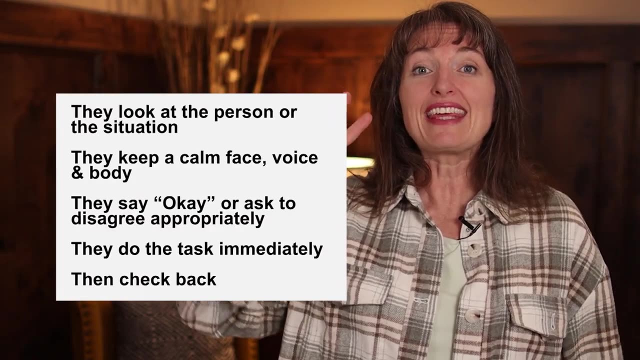 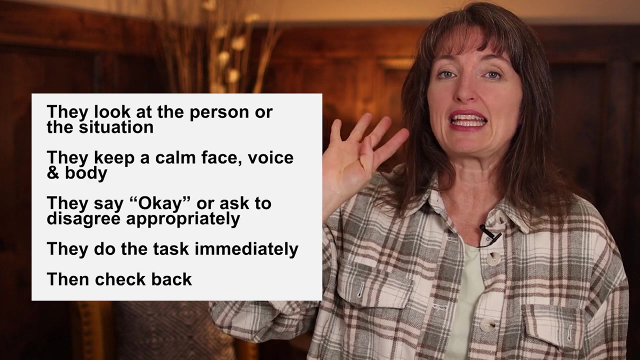 have a time where we practice it the right way again. So let's say, following instructions, for instance, When a person follows instructions, they look at the person of the situation, they keep a calm face, voice and body. They say okay or ask to disagree. appropriately, They do the task immediately and then. 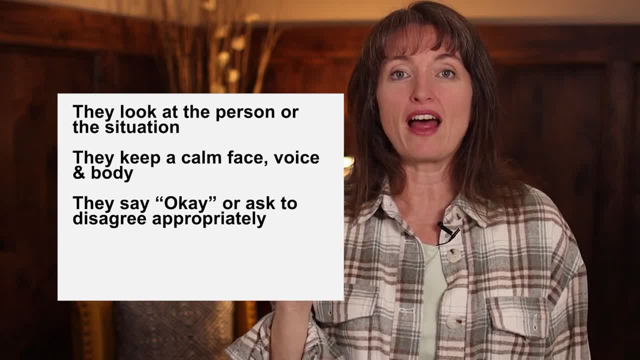 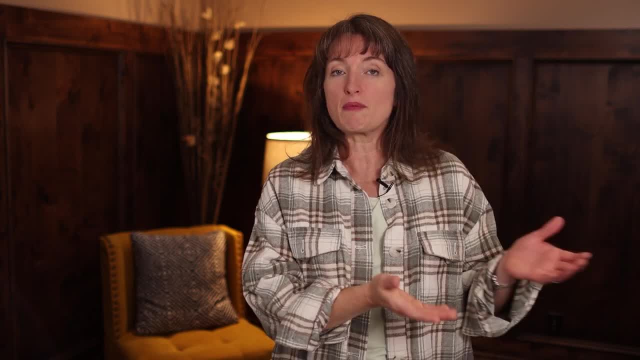 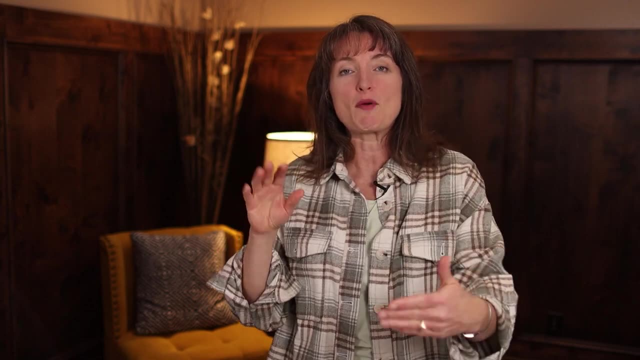 check back. Now. that skill is vital at learning time management, Because at first I am going to give them an instruction to do something with their time. They need to be able to do all 5 of those things and even get back to the check back so that I can praise them When I praise them, and 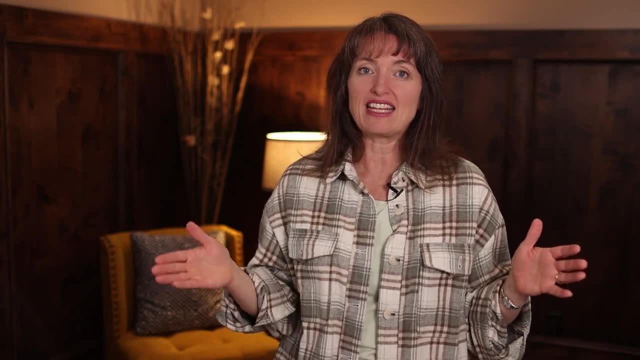 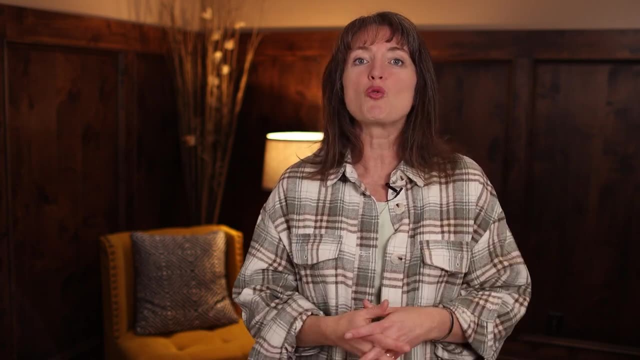 tell them what a great job they did and identify all the things that they did well, then they can duplicate that in the future. If they see cause and effect, they develop a desire to want to follow instructions in the future, And it goes beyond just this. 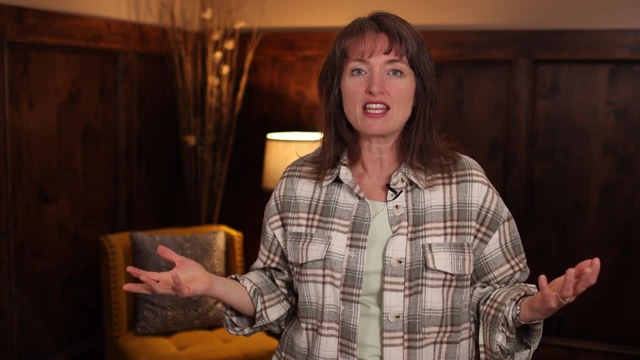 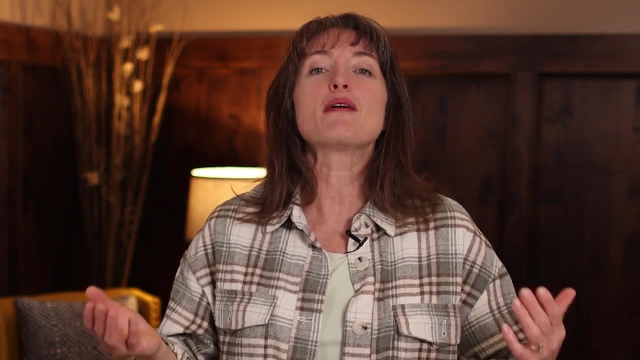 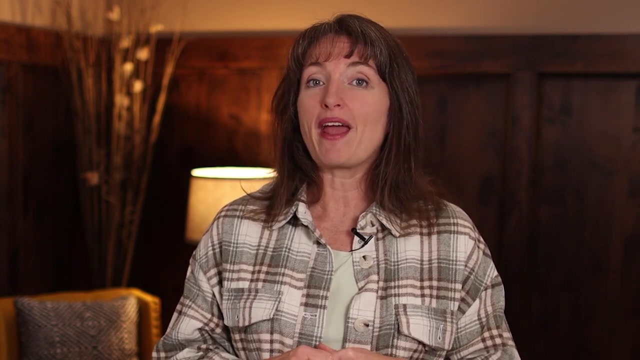 This week or this month. The future is their whole lives. They learn how to follow instruction. They learn also how to give instruction, And a truly self-governed person gives themselves instruction. So soon the children start to learn to give themselves instructions and no answers. So let's talk a little. 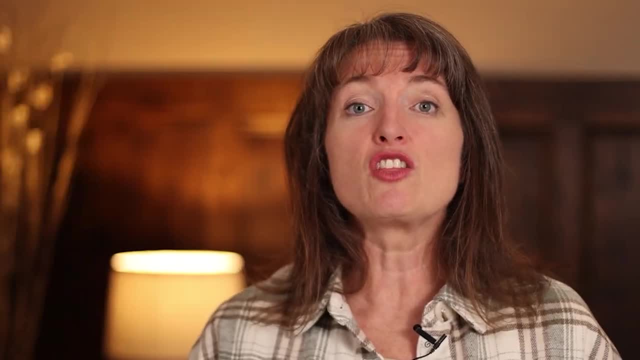 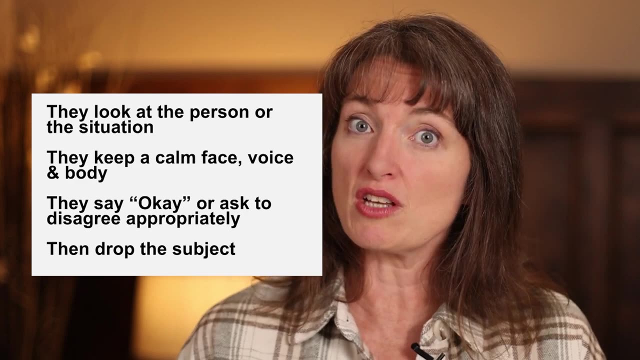 bit about accepting no answers. When a person accepts no answers, they look at the situation or the person, They keep a calm face, voice and body, They say okay or ask to disagree appropriately- which is another one of our skills- And then they drop the subject. So when a person is budgeting, 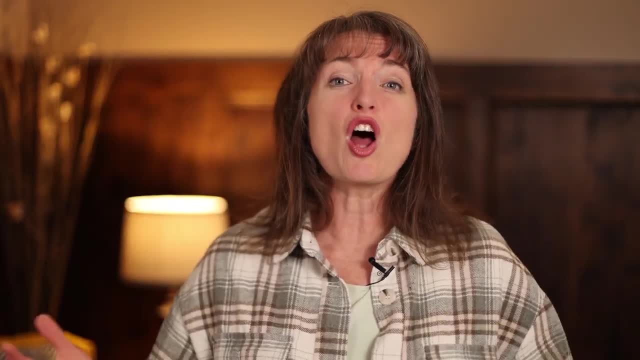 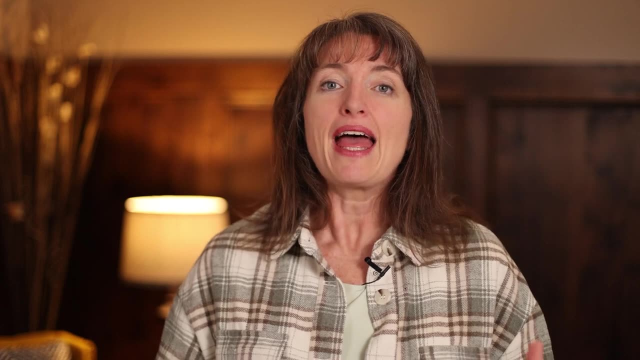 their time. they have to give themselves no answers because there's always going to be distractions. But you can identify those distractions for your children as no answers and tell them and teach them how to give themselves a no answers about their distraction, so that they can stay the course and learn self-government. 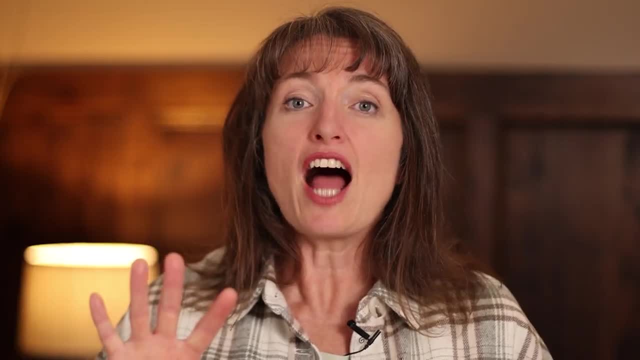 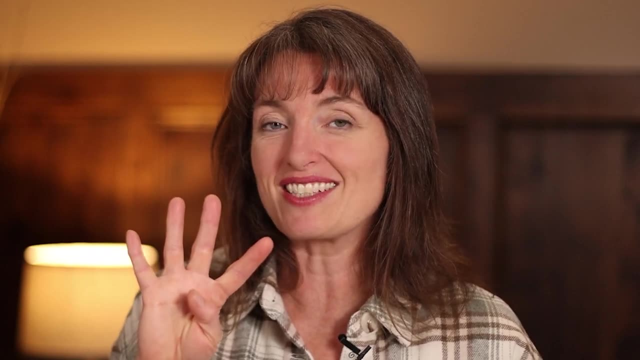 So that's what I did. I taught my children 4 basic skills. I taught them the skill for correction, praise, pre-teaching, so that we can evaluate how they were doing at using their 4 basic skills, And then they followed through. Now I've. 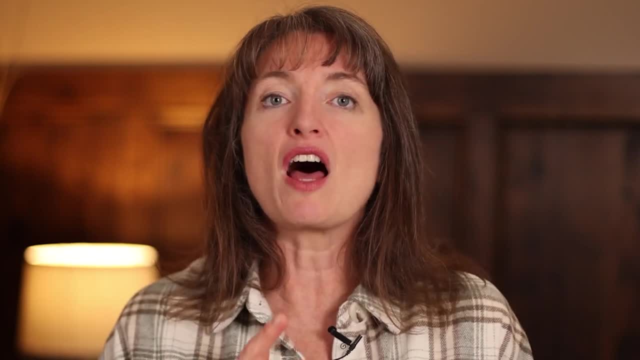 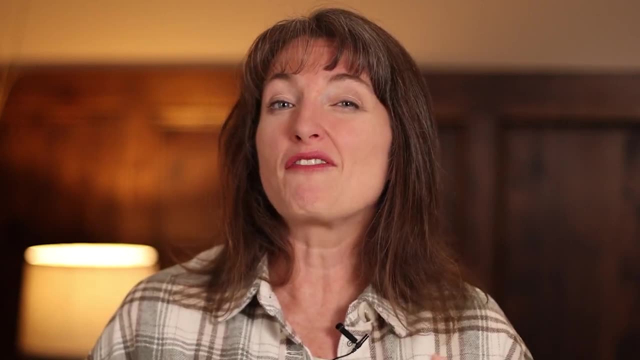 only told you the skill sets for 2 of them, But you can find those other ones on my course or other places. Then they can evaluate themselves By the time they were like 5 years old or 4 years old when we were having our weekly meetings. 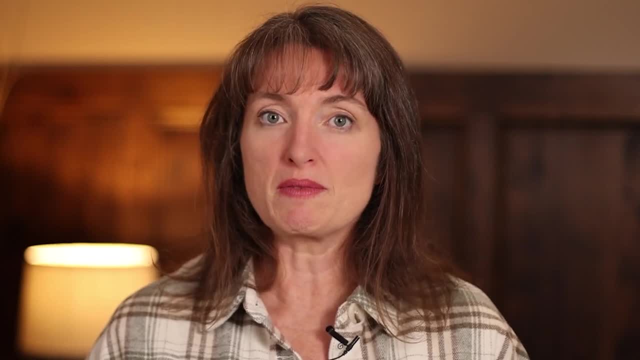 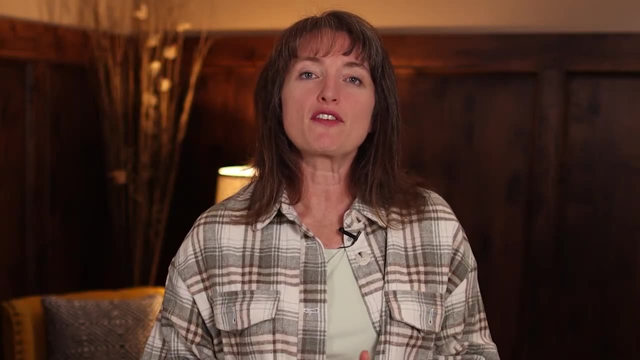 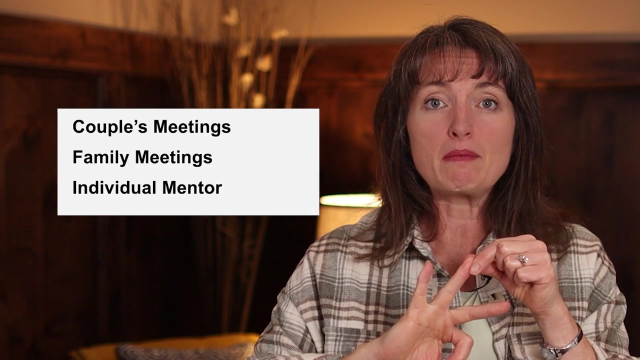 which we call mentor meetings. they started setting goals for themselves and following through This led very naturally into some time management. So in the teaching, self-government, parenting model, we have 3 meetings that we have each week. So there's couples meeting and then family. 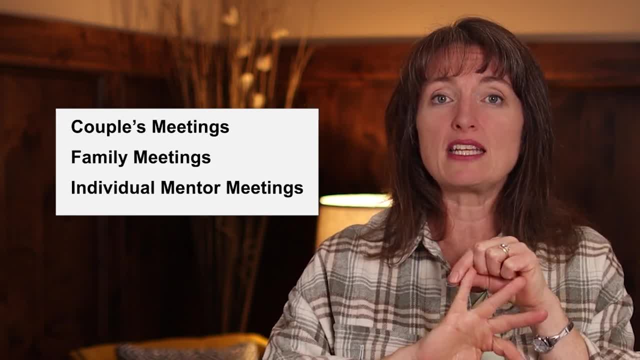 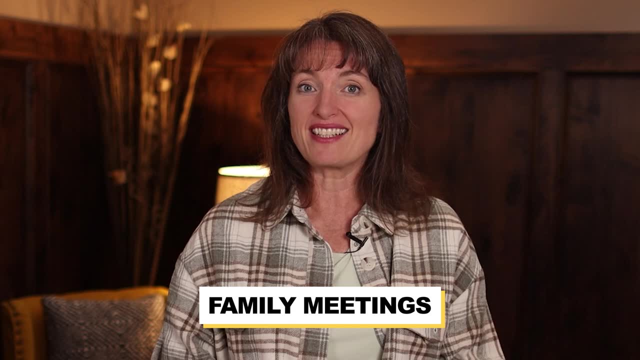 meetings and then individual mentor meetings. So family meetings and individual mentor meetings are what I would like to talk about right now. The family meetings are a great time for everybody to analyze cause and effect as a group and to see how they can approve as a group So they take an active role. 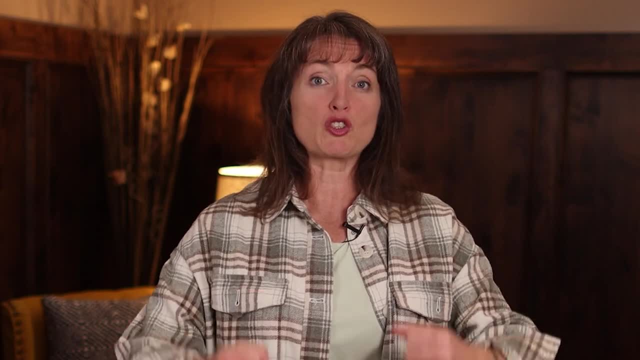 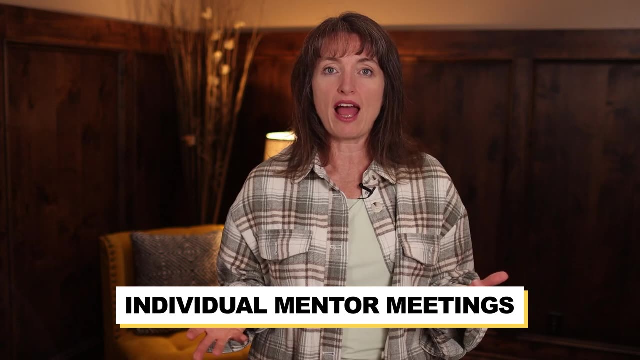 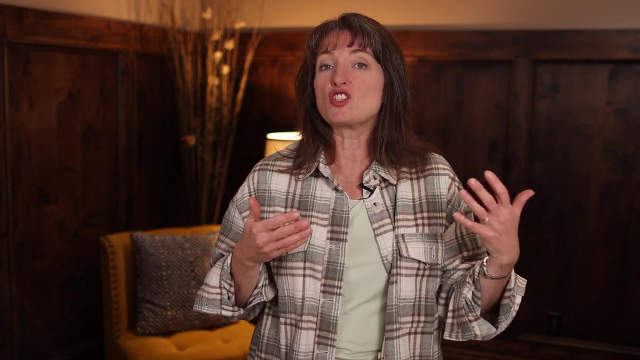 in solving problems as a family. This helps them take personal responsibility for themselves. In the mentor meetings individually, they set goals in different areas of their lives: Personal goals, spiritual goals, academic goals, social goals. They talk about things they want to do for fun, set goals for that And 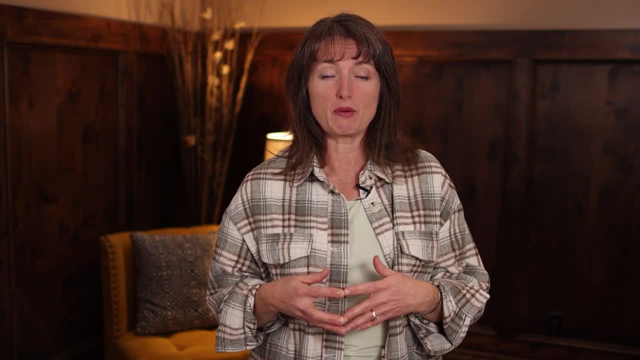 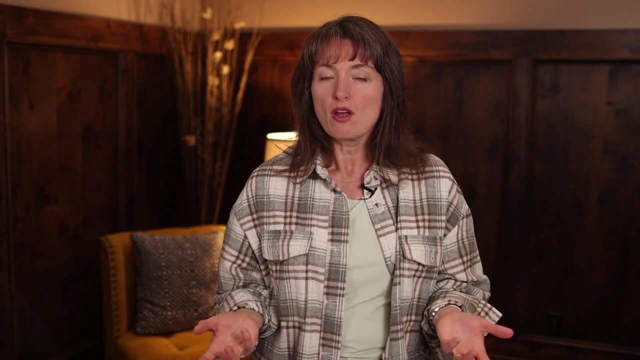 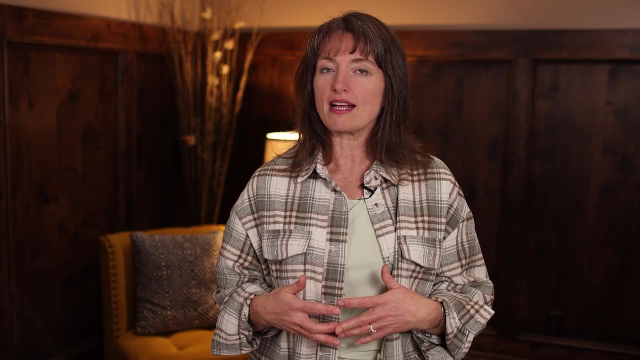 areas of concern that they might have or want to discuss with their parents And set goals for change there as well. So when they are in the habit of setting these goals for themselves, then they also feel a little bit more invested in their own progress. 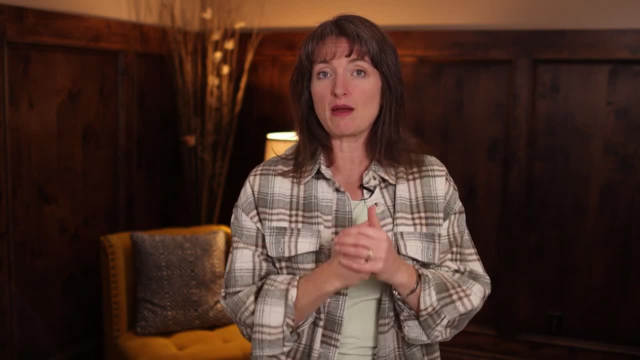 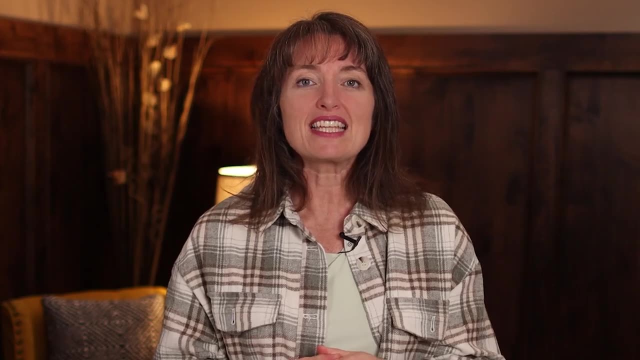 There's also a spot on the forum where we fill out a calendar for them each week So they put key things that they want to do in the days of the week so that they remember to follow through. This gives them practice, starting when they're really young. 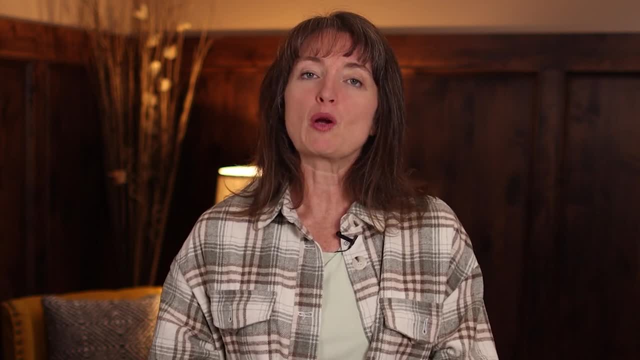 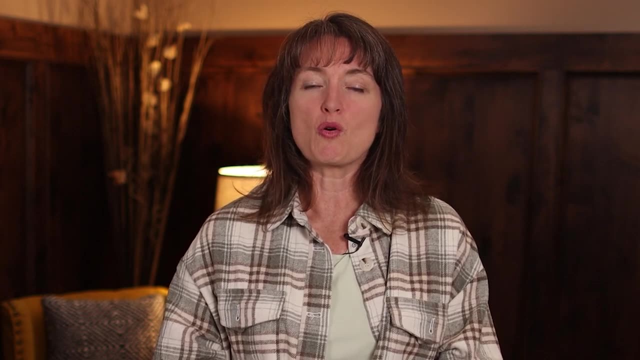 at following through with some of their own goals. When a person learns time management, it's because they set a goal and they follow through. They know how to make themselves stay the course. This takes practice. People aren't going to be perfect at it at first, So it's good to start when they're young. 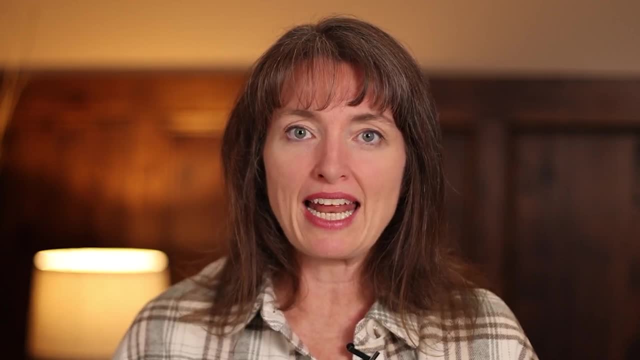 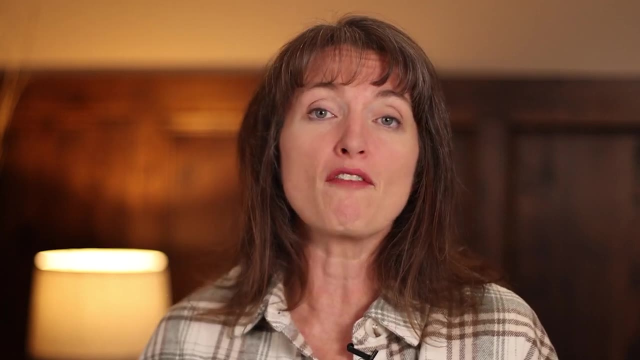 Now, were my children perfect at time management at age 6? No way, But they were pretty good, In fact. I could leave for a full day training somewhere where I was doing a conference and I could leave like a little paper bag with a treat in it. 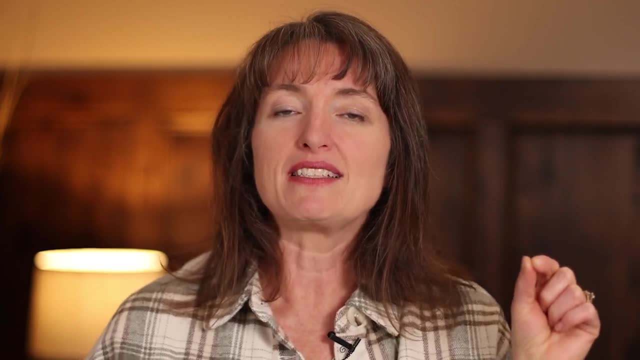 with their name on it and they couldn't see what the treat was. And I would say: okay, as soon as you're done with all of your schoolwork, you need to do this for math because I was a homeschooler. okay. 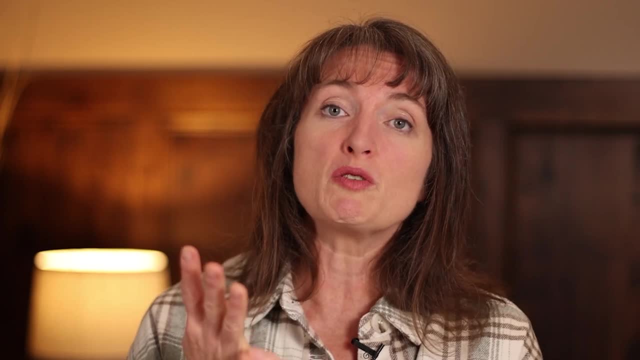 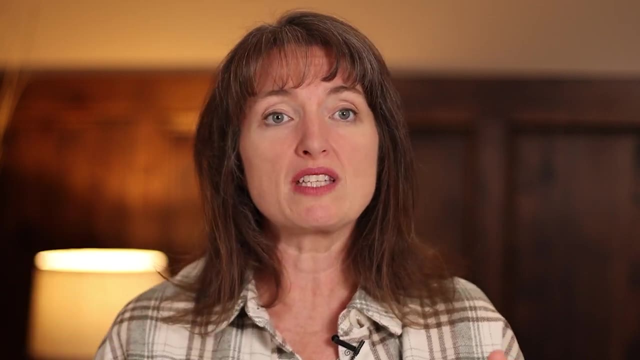 This for math, this for reading. you need to do your chore, your music practice. you know, I would list what they needed to do and put it in a list for them to check off And I would say: as soon as you're done with those things, then you can pick one of the grab bags. 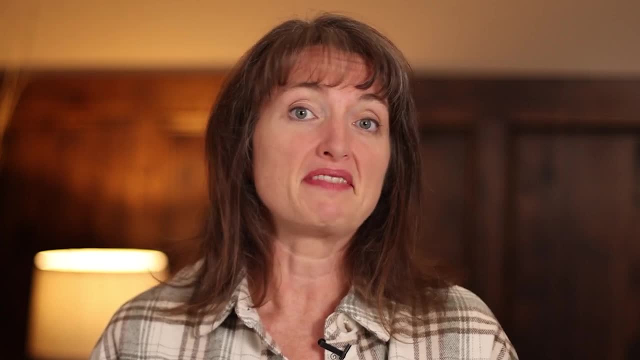 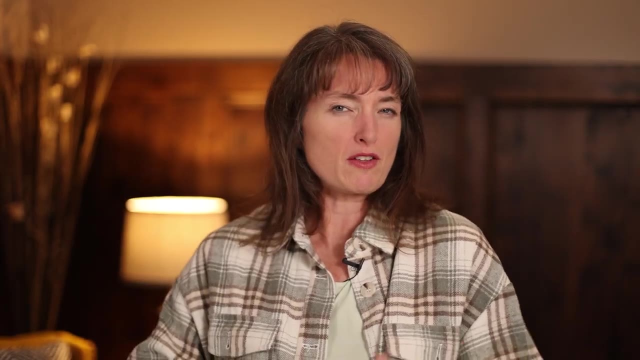 and you can have that for your treat. And guess what? They did it Every time they did it And they did all of their things and they loved doing their stuff alone. They felt so big and grown up No one had to hold their hand or look over their shoulder. They couldn't.